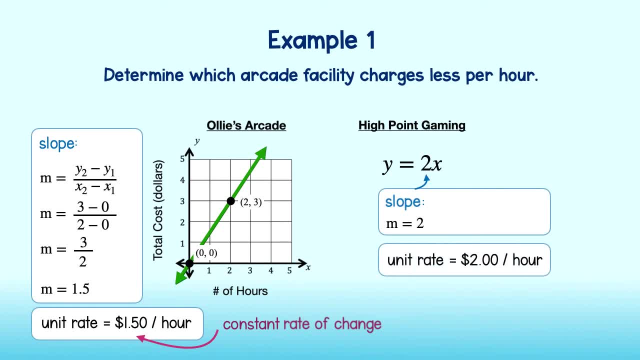 slope is 2, the slope is 1.5.. Since the slope is 2,, the slope is 1.5.. Since the slope is 2, the unit rate is 2, which tells me that High Point charges $2 per hour. If Harley. 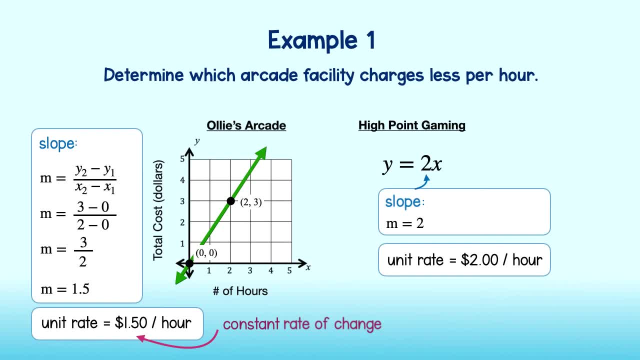 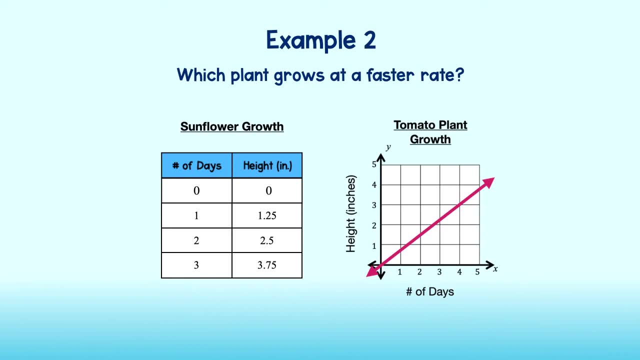 and his friends want to go to the less expensive arcade, they should choose Ollie's Arcade. Let's take a look at another example. Here you will see the data pertaining to the growth of both a sunflower and a tomato plant. We want to figure out which plant grows at a 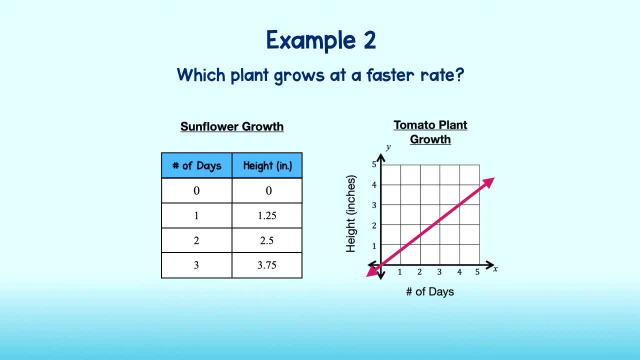 faster rate. So let's see, We are trying to figure out the rate of each plant. Let's take a look at the sunflower. I see that both sets of data show the plant's growth over a period of days. It will be most beneficial if we can find the unit rate or the rate. 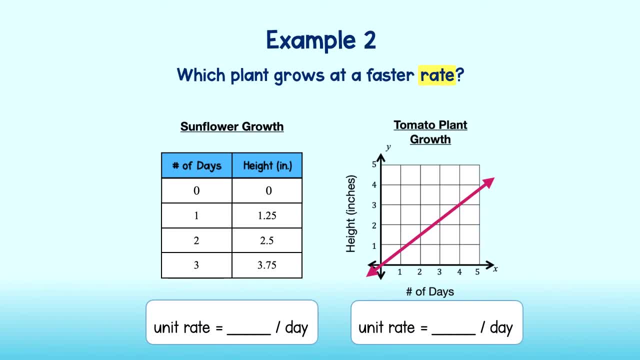 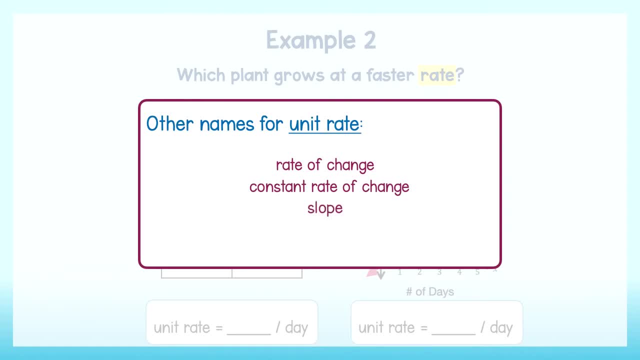 at which each plant grows. per one day, We learned a couple of different names for unit rate, Rate of change, constant rate of change and slope- Yes, slope. If we can figure out the slope of both sets of data, then we can answer the question. Let's take a look at. 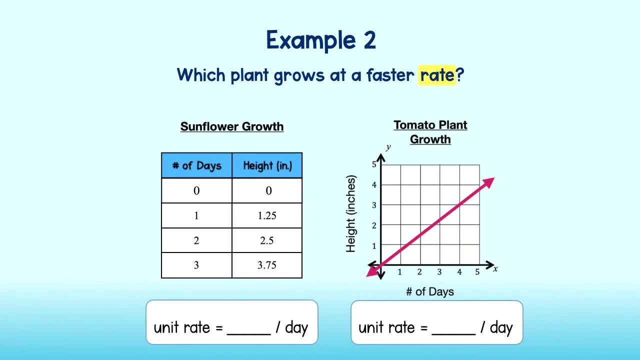 the sunflower. I'm going to write the equation that represents this table because I think it will help me determine the slope. If I multiply each of the x values by 1.25,, I see that I get the corresponding y value. Therefore, my equation is: y equals 1.25x. I see the slope is 1.25,. 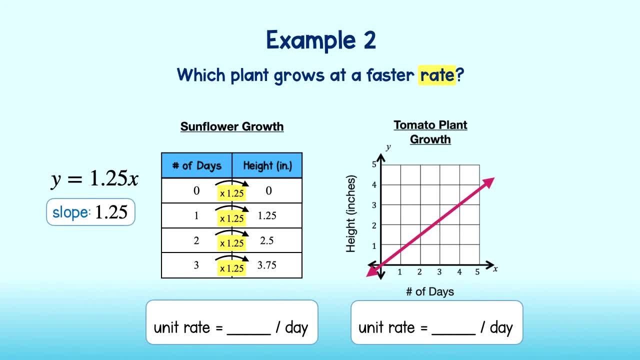 which means the constant rate of change, or unit rate that the sunflower grows is 1.25 inches or 1.25 inches per day. Alright, I want to know how many inches the tomato plant grows in one day. To do that. 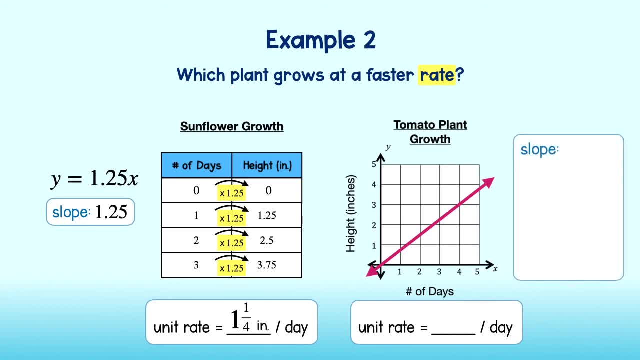 I will calculate the slope. Slope or m is equal to y2-y1 over x2-x1.. I will choose the point which will represent x1 and y1, and which will represent x2 and y2.. Then 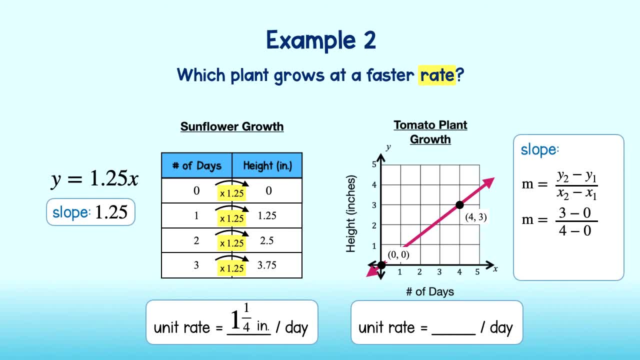 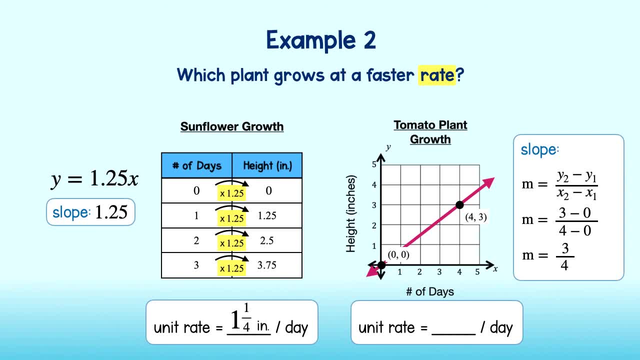 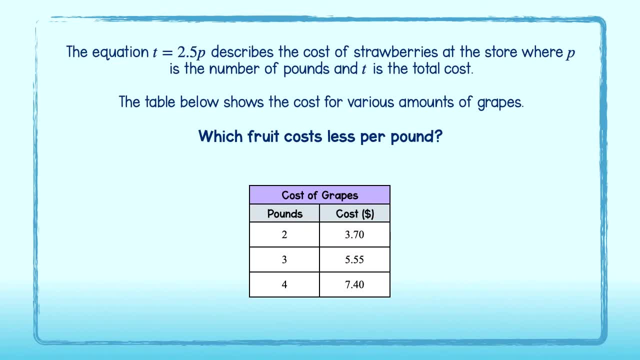 a much faster rate than the tomato plant. Okay, your turn. The equation T equals 2.5p describes the cost of strawberries at the store, where P is the number of pounds and T is the total cost. The table below shows amounts of grapes. Which fruit costs less per pound? Take a minute and try to. 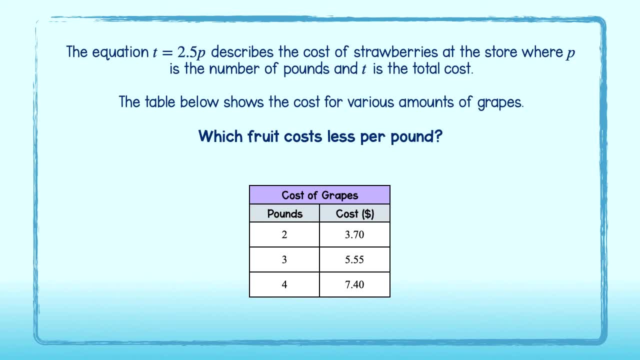 figure this one out. Remember to pause the video for more time. Okay, before we start, let's address the equation. t equals 2.5p. here in the problem, You might have noticed the different variables t and p. That is okay. 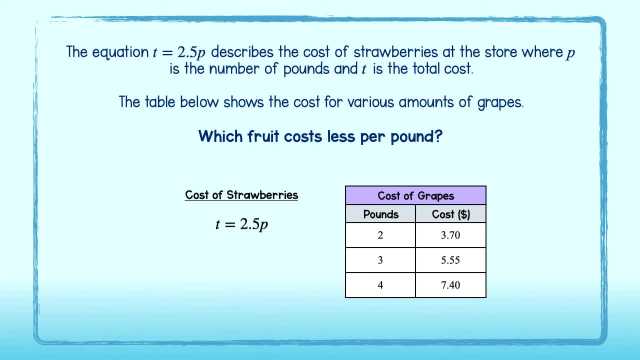 It is still in the form of y equals mx and will still give us the same information. They're just a little more specific in that the problem is using t for total cost and p for pounds. Okay, looking at this equation, however, we see: 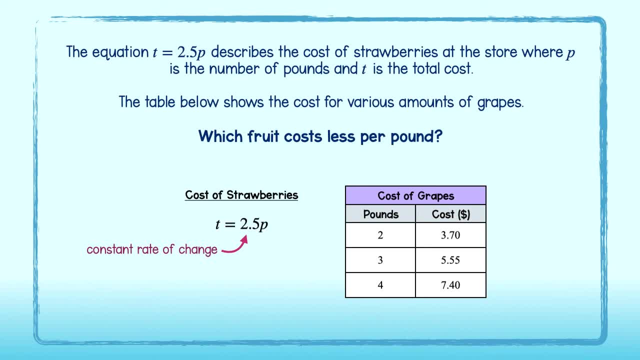 the constant rate of change is 2.5.. This tells us that the unit rate is two dollars and fifty cents per pound of strawberries. Now let's take a look at the table. I know if I can write the equation that represents the table then. 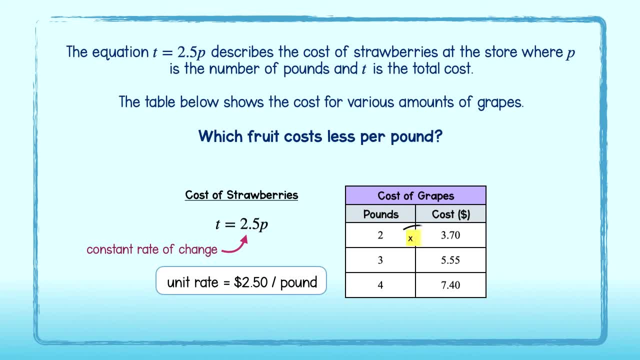 I can identify the unit rate. What can I multiply by Each of my x values by to get the corresponding y value? Well, if it's not apparent, we can use the inverse operation, or, in this case, division, to quickly figure it out: 3.70 divided by 2 is equal to 1.85.. The same is true for: 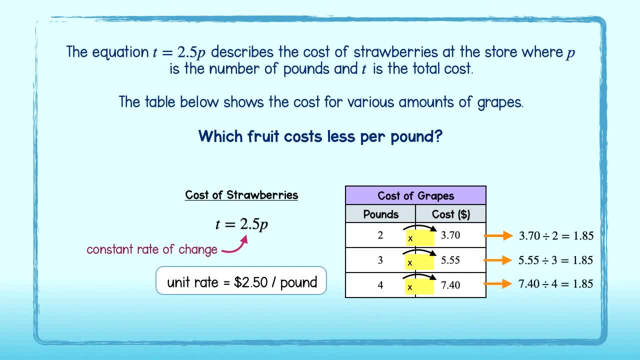 the rest of the values. This means that if I multiply the x values by 1.85, then I will get the corresponding y values. 1.85 is the constant rate of change and therefore my equation is: y equals 1.85x and the unit rate for the cost of grapes is one dollar and eighty-five cents per pound. Comparing the two prices, I see that grapes cost much less. Nice work. Thanks for watching.